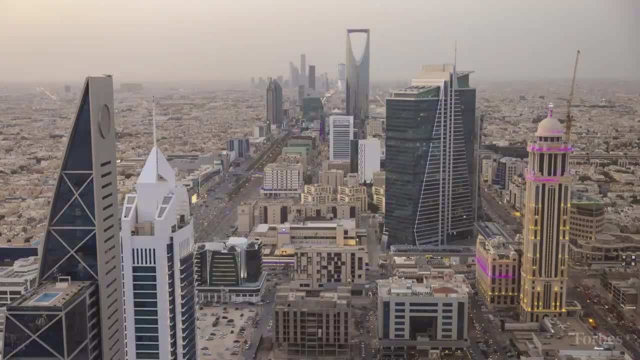 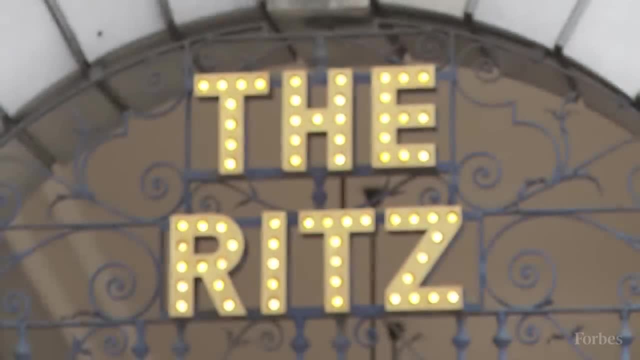 The desert is a place where you can see the desert from the sky. The desert is a place where you can see the desert from the sky. Then there are all the new hotels, with their thousands of freshly built rooms, The world's most iconic hospitality companies: Ritz-Carlton, Four Seasons, St Regis, Fairmont, Marriott. 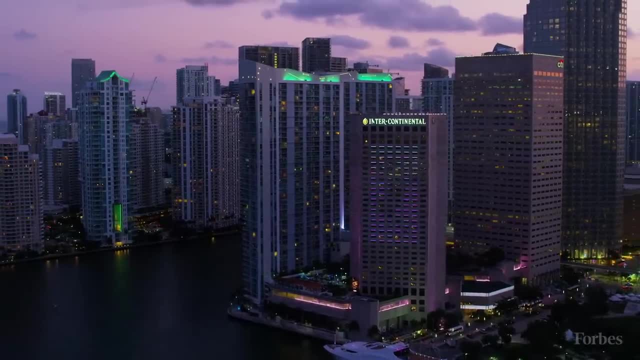 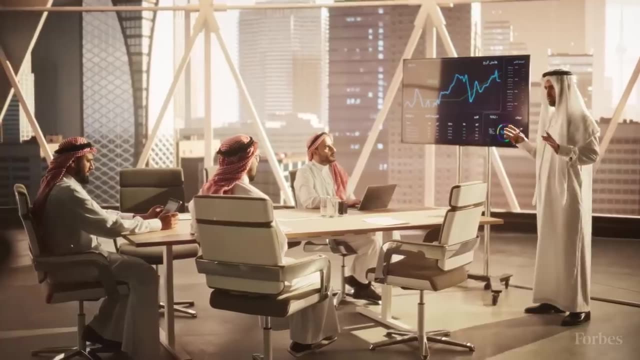 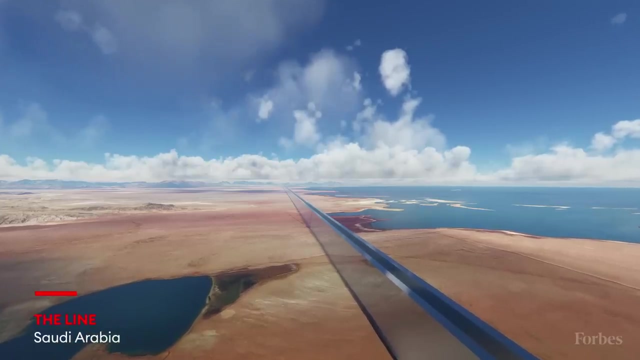 Hilton, Hyatt and Intercontinental are falling over themselves to jump into a construction pipeline that's churning faster than anywhere else in the world. Any one of these projects might momentarily pierce the travel industry, But together, what's going on in Saudi Arabia simply cannot be ignored. 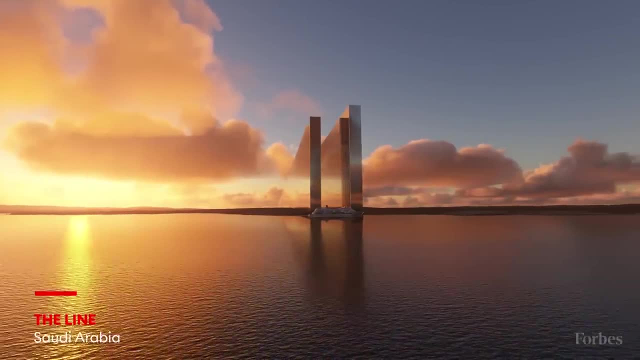 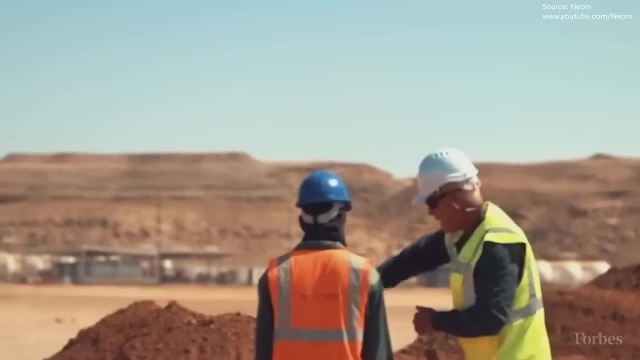 It can be difficult to visualize the vastness of Saudi Arabia's physical transformation. Some of the most notable ongoing projects fall within NEOM, a $500 billion built-from-scratch region in northwest Saudi Arabia where the kingdom is creating new cities, resorts and. 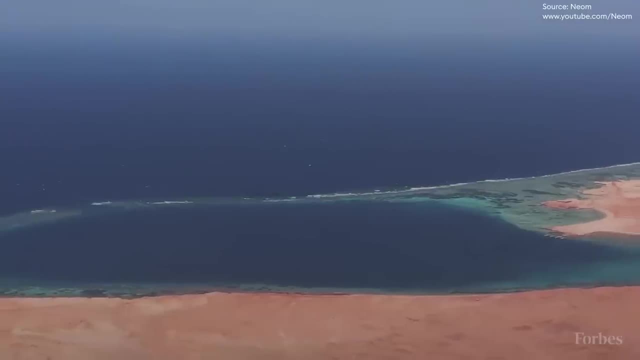 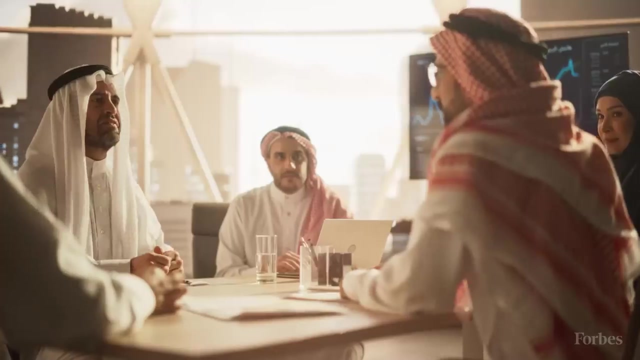 other developments. At 10,200 square miles and bounded by the Red Sea to the south and the Gulf of Aqsa Aqaba to the west, it's roughly the size of Albania. Bankrolled by the kingdom's $700 billion public investment fund, the idea for NEOM was born. 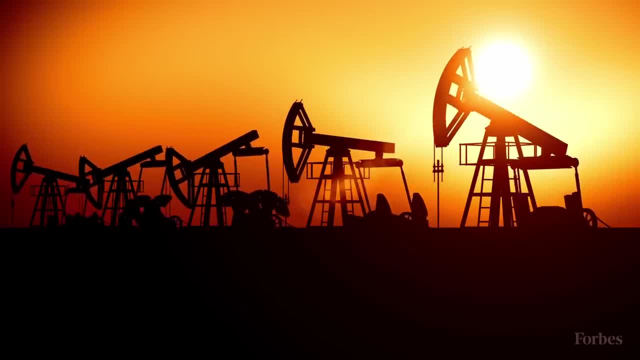 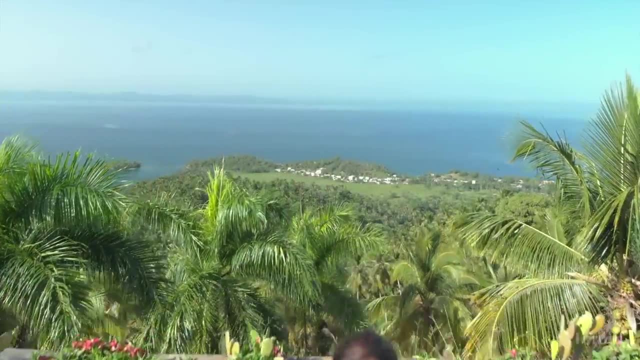 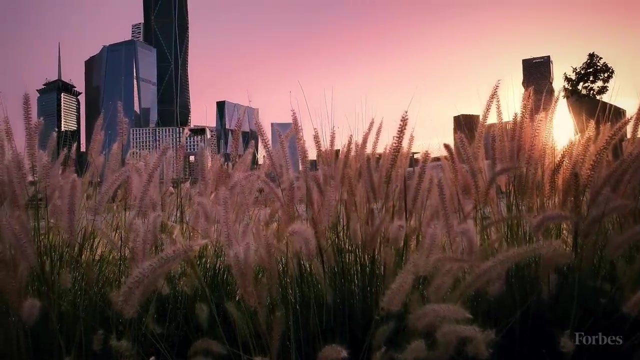 out of Vision 2030, Saudi Arabia's grand plan to shake off its historic reliance on oil and diversify its economy. One of the scheme's pillars involves reinventing the country as a global tourism juggernaut. When first announced in 2016,, the kingdom's tourism goals seemed fanciful: Attract $100. 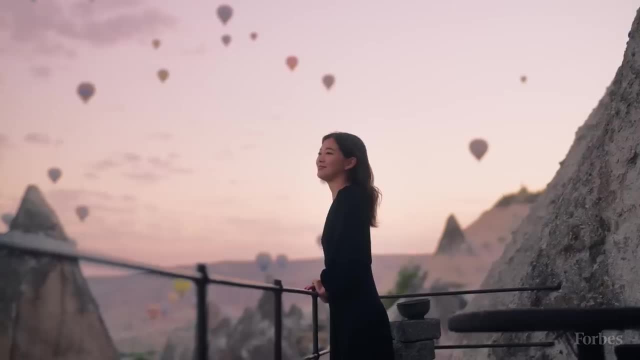 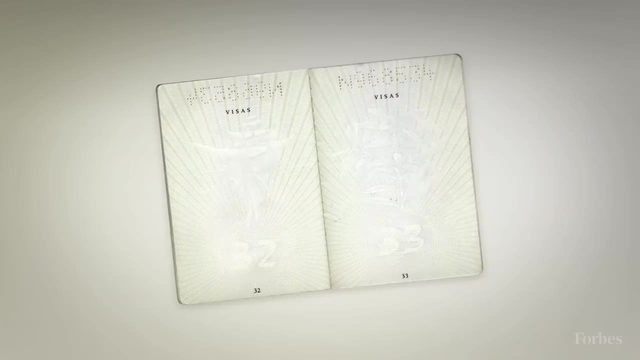 billion of foreign and domestic visitors to the country every year and grow tourism's share of the economy from about 3% to 10%, and do it all in just 14 years. Then, in 2019, Saudi Arabia announced it would provide e-visas and visas on arrival to visitors. 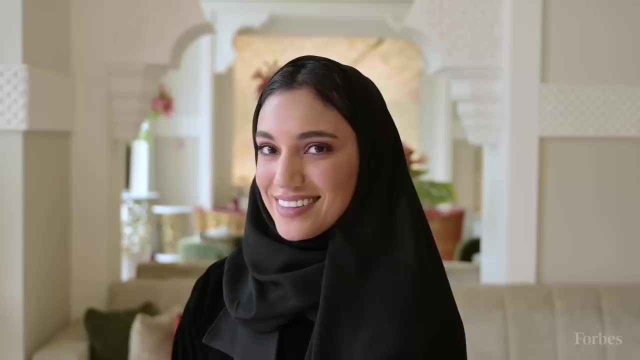 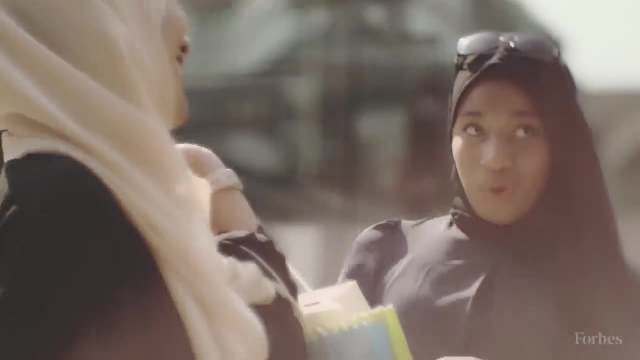 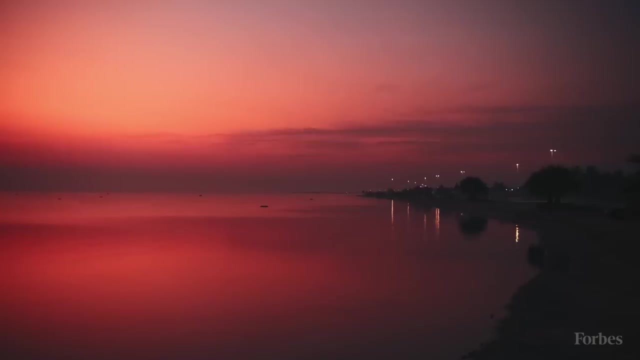 from 49 countries, including the United States. Among other changes announced at the time, female visitors would be exempted from wearing an abaya, the traditional and otherwise obligatory head-to-toe robe in public places, and would be allowed to travel without a male companion. 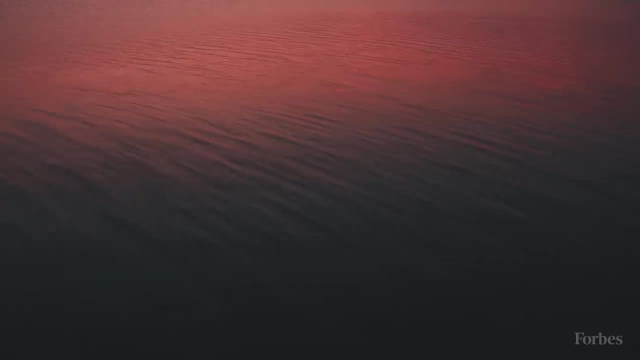 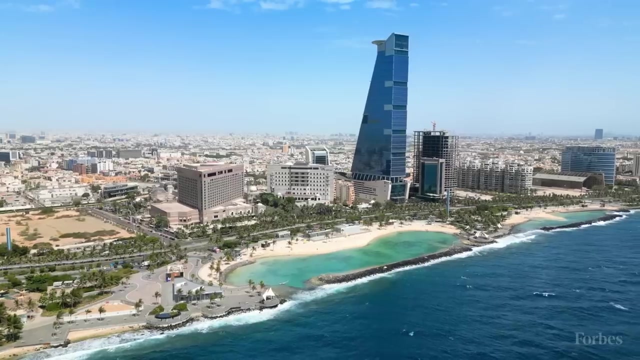 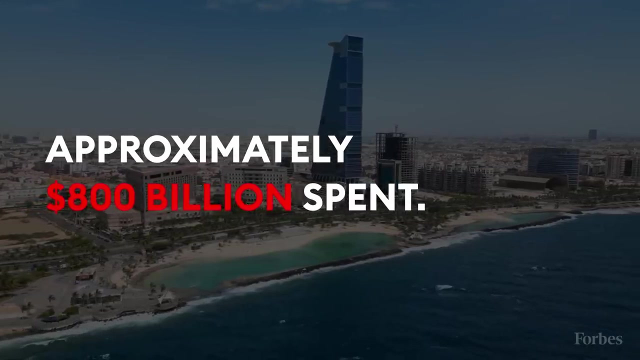 Since Saudi Arabia opened to the international travel market, the speed and spare-no-expense approach to its transformation has stunned even the most seasoned tourism analysts. The World Travel and Tourism Council estimates the kingdom has already spent $800 billion, and that doesn't include the massive amounts of foreign investments pouring in. 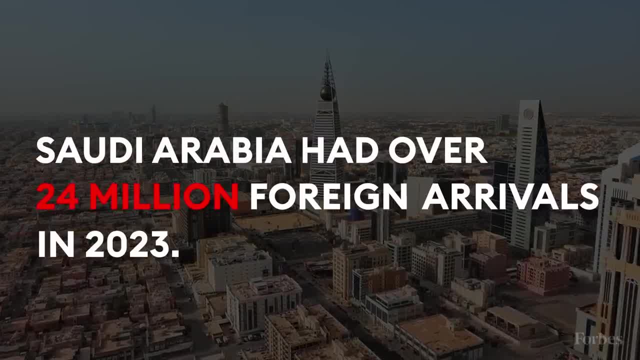 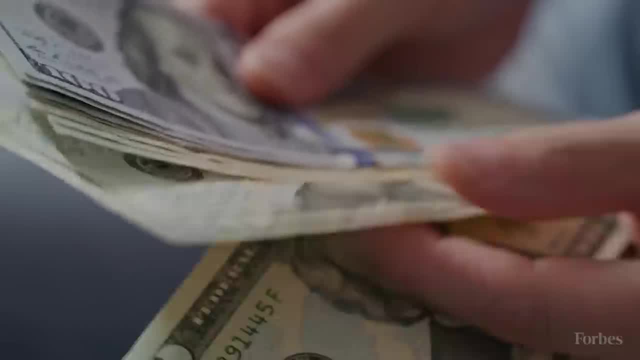 Saudi Arabia had over 24 million foreign arrivals in 2023, and will welcome nearly 37 million in 2030,, according to Euromonitor projections. A more meaningful measure of success is how much foreigners are expected to spend while in Saudi Arabia. 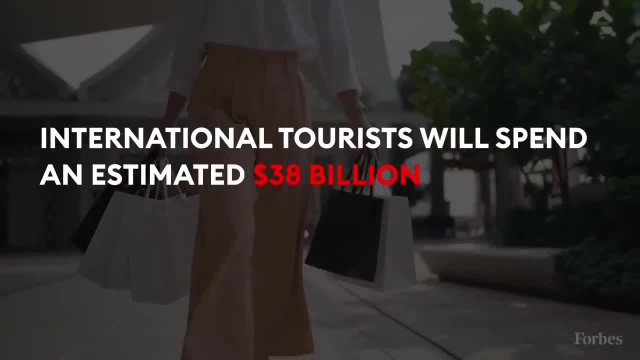 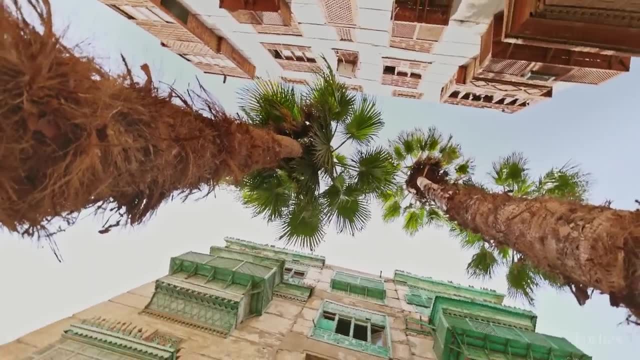 Euromonitor predicts that international tourists will spend $38 billion in 2030. But the total economic impact for Saudi Arabia will be far greater. after adding in domestic travelers' expenditures and the ripple effect of 1 million new tourism jobs, The WTTC projects that by 2032, the total economic impact of Saudi Arabia will be much. 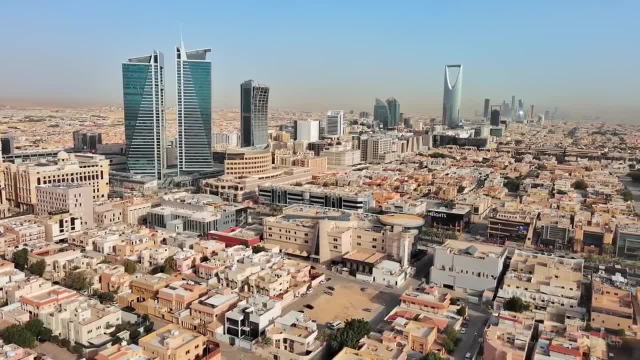 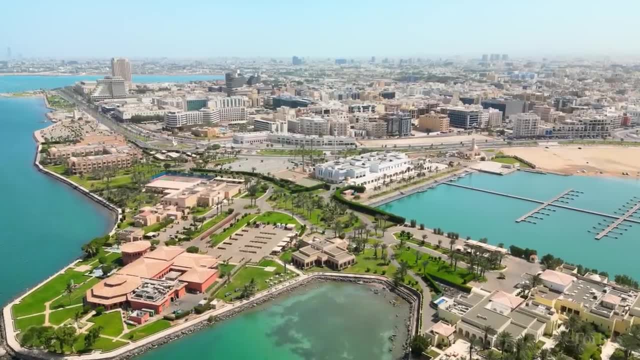 greater than the total economic impact of Saudi Arabia. In 2022,, Saudi Arabia's tourism sector could contribute nearly $169 billion to its GDP, representing 17.1% of the total Saudi economy. Preparing for the future also means recognizing the seismic shift in what the next generations 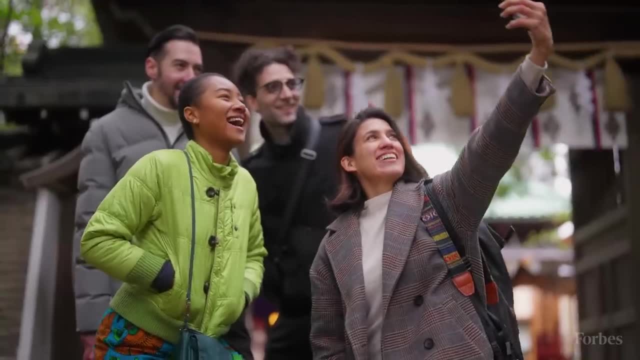 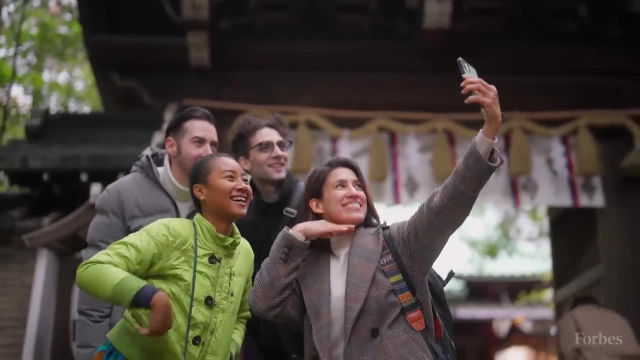 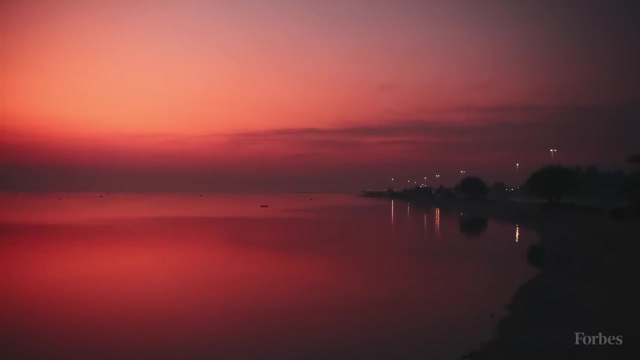 of global travelers will want. Roughly 90% of young Chinese travelers and 70% of Gen Z travelers in the UK, Australia and India say they are looking to discover new destinations, according to data from Skift Research. In that sense, being the new kid on the tourism block is an enormous plus. 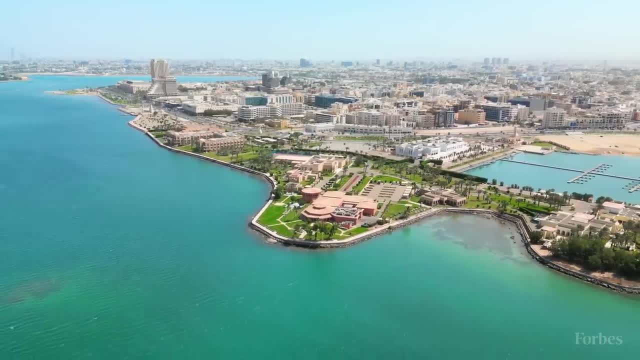 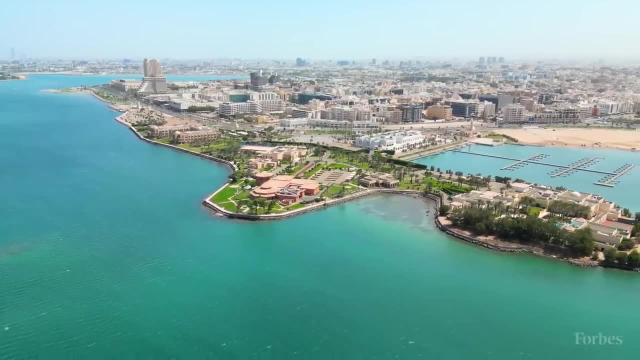 There are, of course, many ways for the Saudi grand vision to go sideways. First, there are enormous financial risks inherent in tackling so many giga projects all at once, even for a country with bottomless pockets. The kingdom's debt-to-GDP ratio is nearly double what it was a decade ago, though still. quite low compared to other countries. Another concern is hotel overcapacity. The United Kingdom's debt-to-GDP ratio is nearly double what it was a decade ago, though still quite low compared to other countries. Another concern is hotel overcapacity. The US past model predicts that the average traveler's spend will have already dropped. 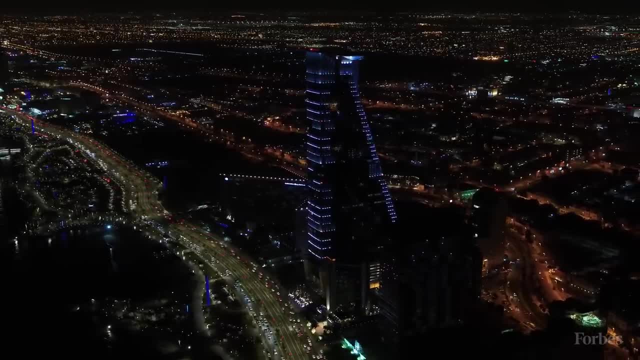 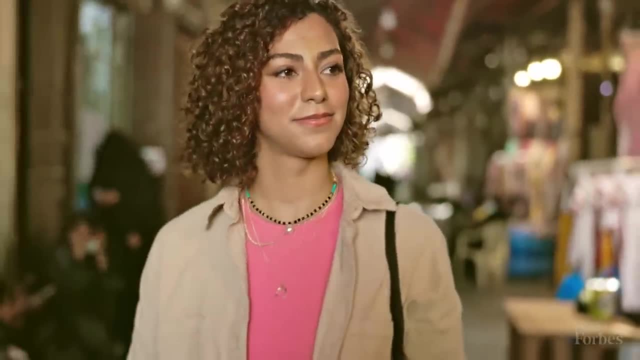 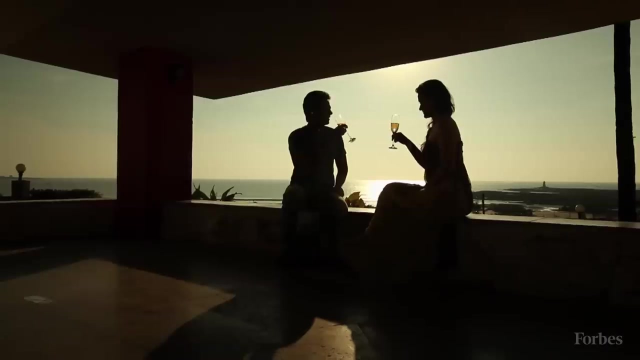 by 2030.. Too many hotel rooms that aren't being filled would drive prices down. In addition, Saudi Arabia has a persistent PR problem among many would-be travelers, especially those from the West. The kingdom still has strict laws about drinking and severe restrictions for women not to. 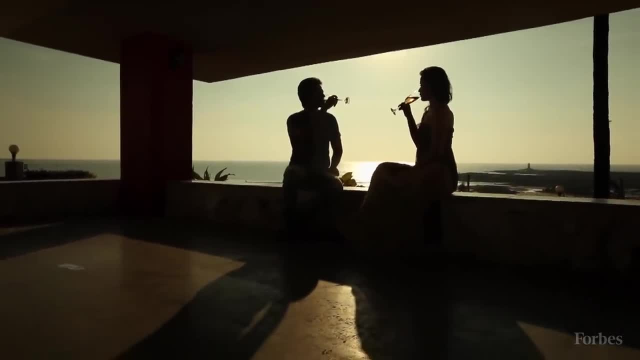 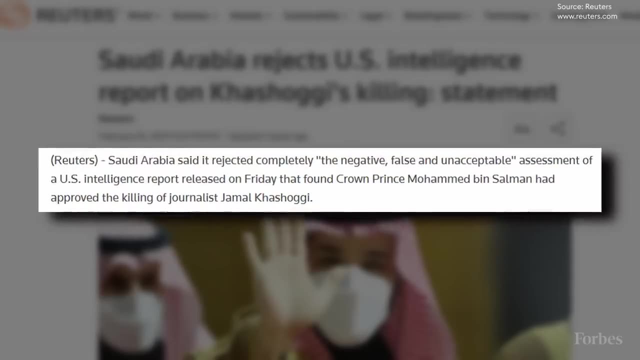 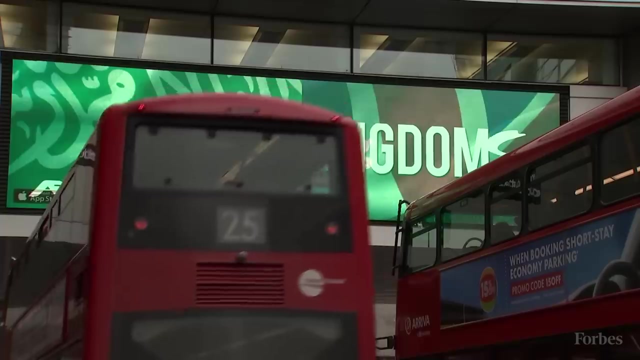 mention allegations of human rights abuses and attacks against journalists. In 2021, the US officially blamed Saudi Crown Prince Mohammed bin Laden for the global threat of the 2018 murder of Washington Post journalist Jamal Khashoggi. But any concerns about human rights haven't stopped multinational corporations from investing.